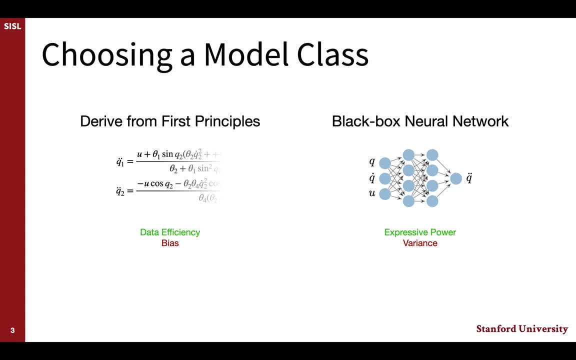 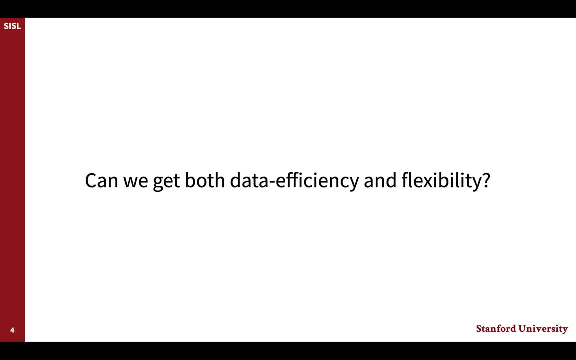 that might be present in the training data. we typically require a lot of training data in order to generalize well, So these models suffer from model variance. So the question we ask is: can we get both the data efficiency of first principle models as well as the flexibility of neural networks? We study a model class that we call structured. 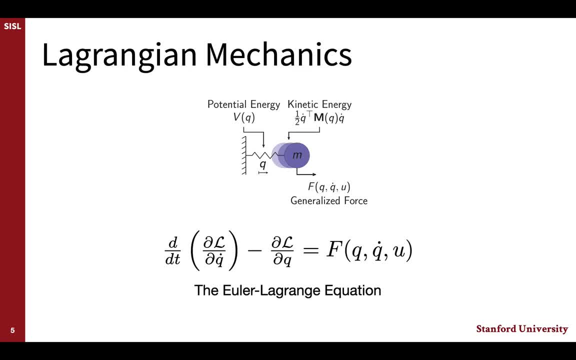 mechanical models. The key insight here is that all mechanical systems obey Lagrangian mechanics. That is to say that if you were able to characterize the potential energy of the system, its kinetic energy, as well as the forces that were acting on it, 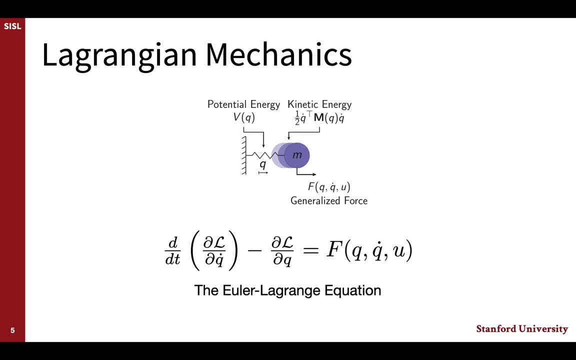 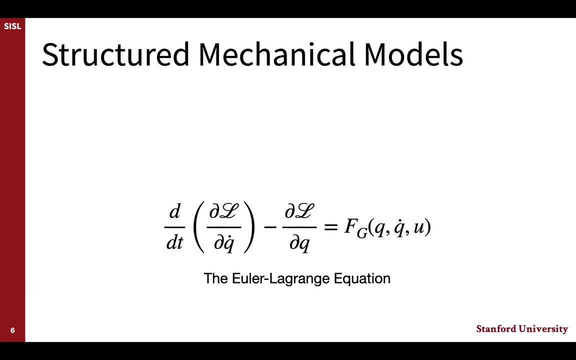 then you could relate these terms through the Euler-Lagrange equation in order to get the system's equations of motion. So what we do is, instead of using a neural network to directly predict data, we use a neural network to directly predict data. So what we do is, instead of using a neural network to directly predict data, 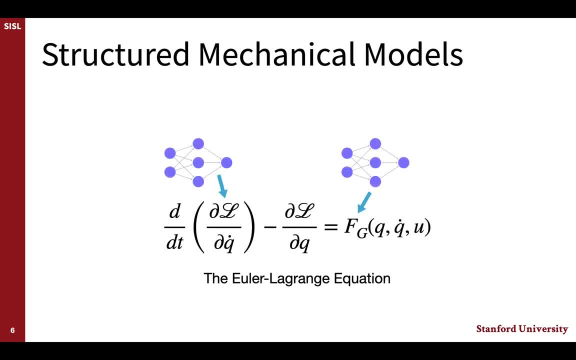 accelerations. we use neural networks to predict the terms of the Euler-Lagrange equation, That is, we predict the system's mass matrix for its kinetic energy, we predict its potential energy as well as the forces that act on it, and we derive the equations of motion through the Euler-Lagrange equation. 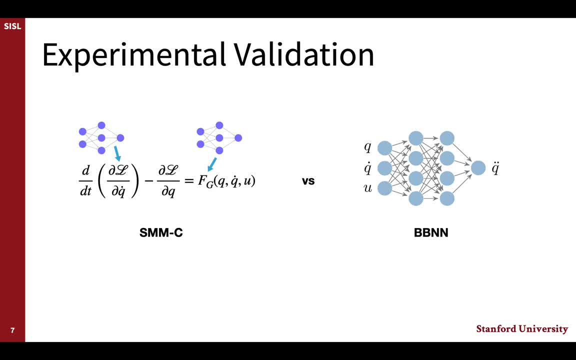 So in experimental validation, we compare the structured mechanical model and we restrict our attention to control affine systems, hence SMMC's, and we compare this to black box neural networks in terms of their ability to generalize from limited data as well as their ability to be used in optimal control. 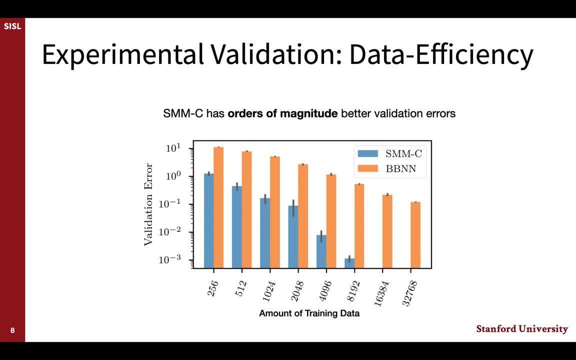 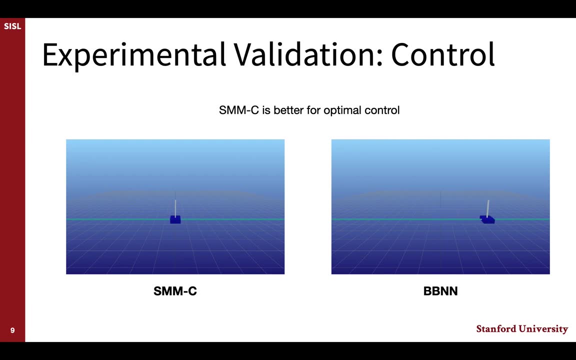 So in terms of data efficiency, we find on a multitude of robotic domains that for the same amount of training data, a structured mechanical model has orders of magnitude better validation error. When we use two models that have the same validation error on an optimal control model, we find that, for the same amount of training data, a structured mechanical model has orders of magnitude better validation error. 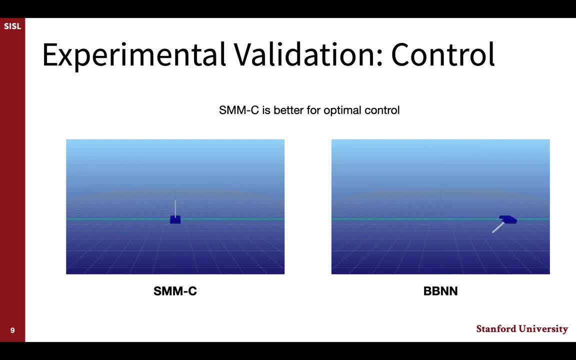 When we use two models that have the same validation error on an optimal control task, we find that structured mechanical models are able to faithfully solve the optimal control task, whereas black box neural networks are not able to do so, And we show that the reason for this is that, even though these two systems are able to get 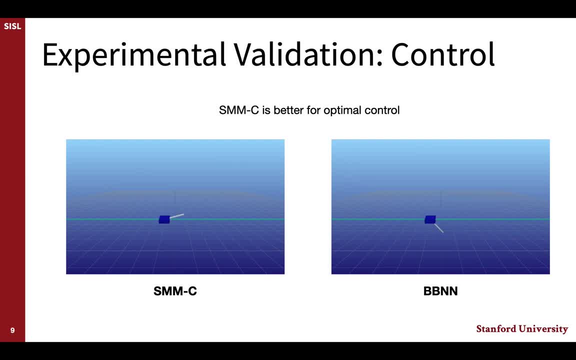 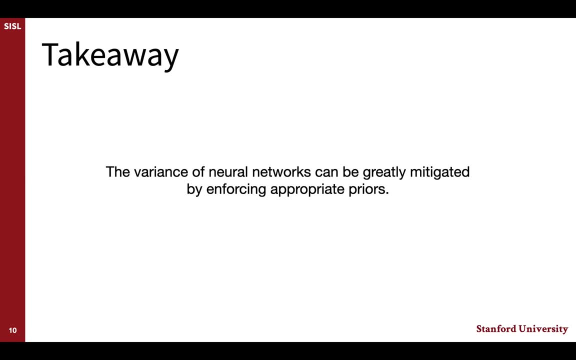 the same validation errors. structured mechanical models give more accurate predictions of the Jacobians. The one sentence takeaway here is that the variance of neural networks can be greatly mitigated by enforcing appropriate priors. We study mechanical systems, and so the appropriate prior to use is Lagrangian mechanics.